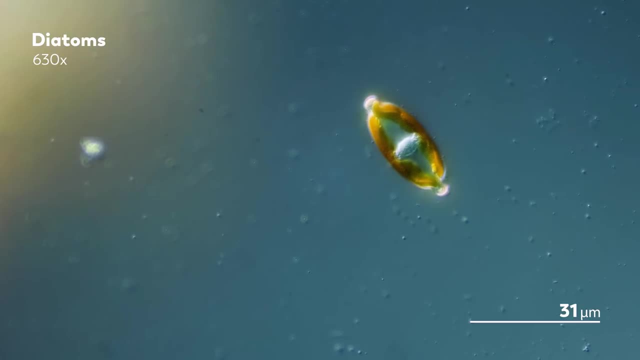 over 70 episodes of Journey to the Microcosmos, but also with her PhD in biomedical engineering and as a host on Crash Course Organic Chemistry. I could not be more excited to have her join me on this journey. So now I'm going to hand the microphone over to Deboki. 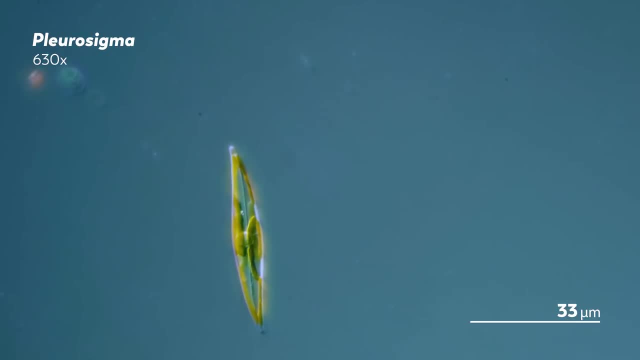 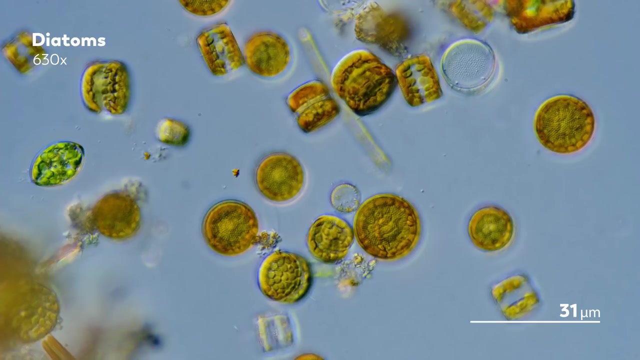 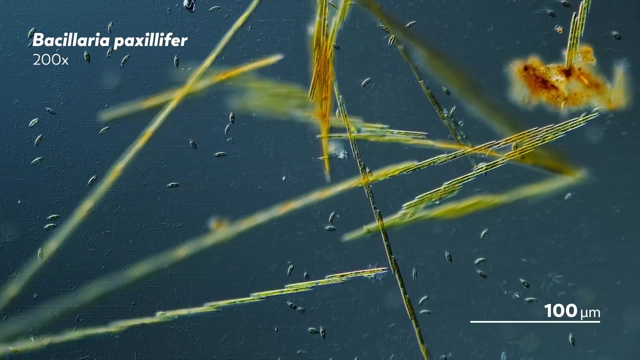 so she can teach you more about diatoms. Wherever you are on your journey to the microcosmos, the odds are high that you'll run into a diatom. They're both abundant and easy to spot because of the shells they encase themselves in. The results are beautiful, exacting geometries that create a living kaleidoscope. 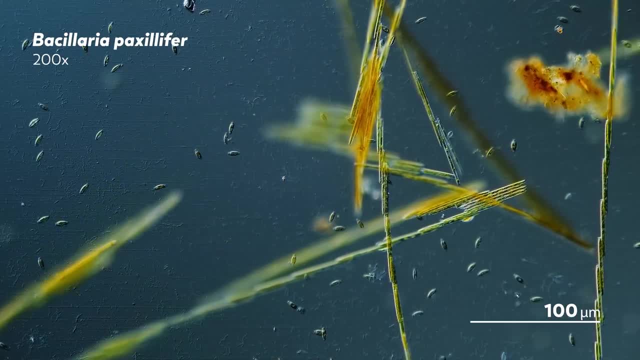 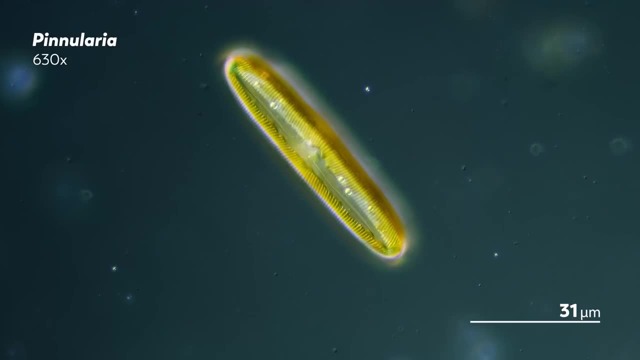 in the microcosmos, And even if you lived your entire life without ever seeing a diatom, without ever hearing the word diatom, you would still be living a life that's shaped by them, all the way down to the oxygen you breathe, Thanks in no small part to their 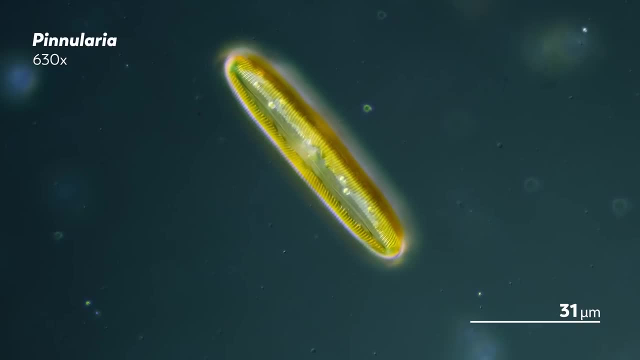 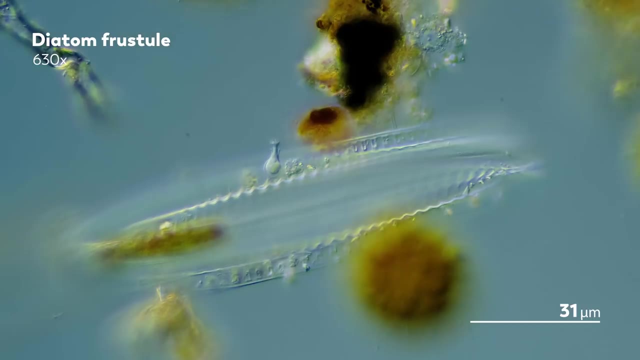 outsized contribution to the world's photosynthesis. But what remains captivating about diatoms is, well, the thing that remains even when the diatom itself is gone: The hard silica shell they once lived in, also known as the frustule. 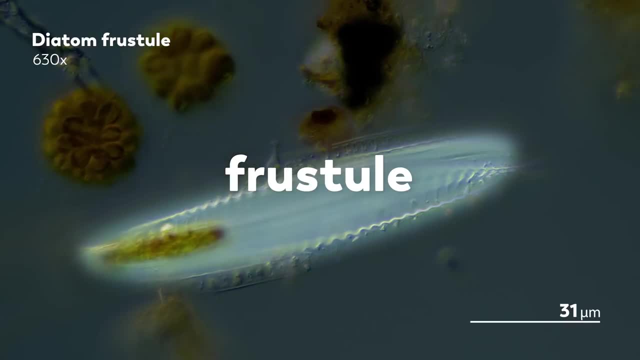 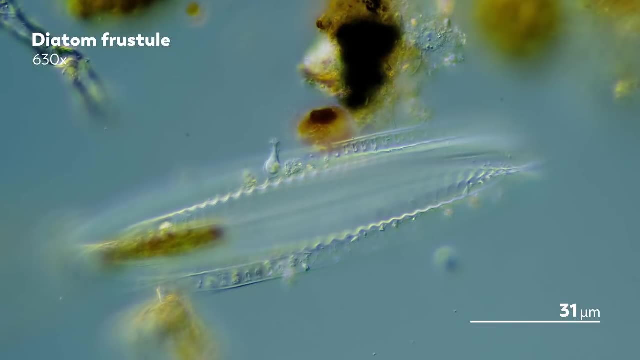 We've talked about frustules a bit before and how they've given diatoms the nickname jewels of the sea, And today we're going to dive a bit more into how those frustules are made and the role they play in our world. 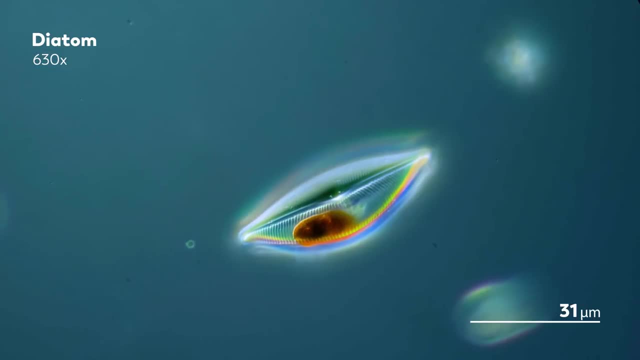 Diatoms are the architects of their own glass houses, And the scale of this project is immense. The silica shells aren't just a smooth, uniform exterior. There are pores and elongated channels, creating ornate microscopic patterns that the organism depends on to survive. 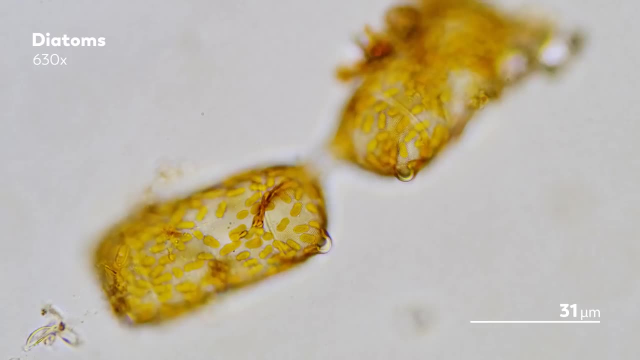 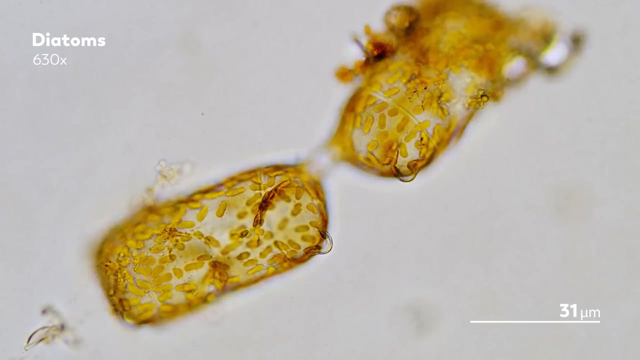 The source of the diatom's building blocks is geology. As rocks and land get weathered and eroded, silica enters the water, where it dissolves into silicic acid, which can then diffuse into the diatom and get converted into silicon. 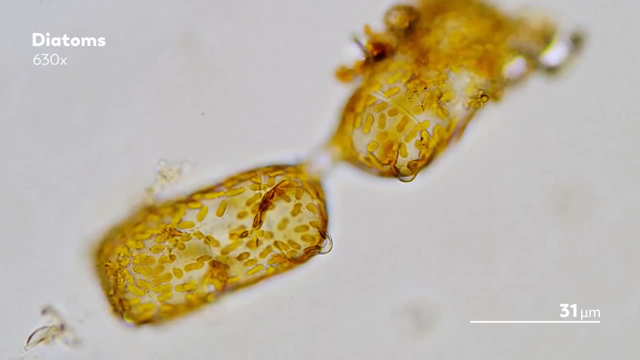 The diatom is the source of the diatom's building blocks. As rocks and land get weathered and eroded, silica enters the water, where it dissolves into silicic acid, which can then diffuse into silica. But if diffusion isn't bringing in enough material, the diatoms can also rely on silicon. 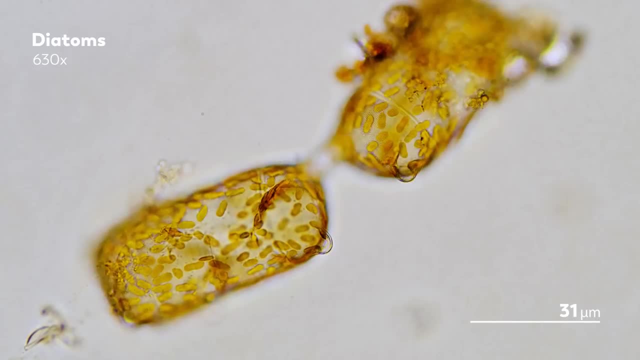 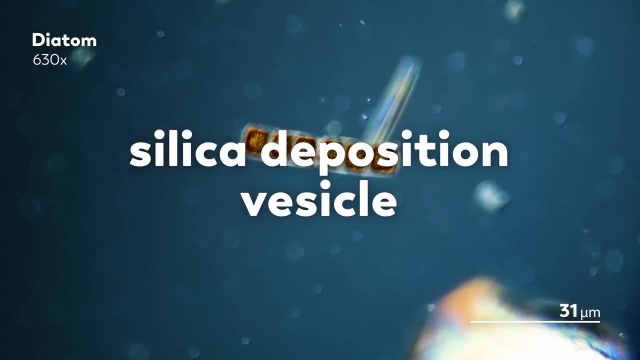 transporter proteins in their membranes. to gather more Inside, the diatom is a special area called the silica deposition vesicle, And it's there that the silica bits get linked together to form bigger and bigger pieces. But while we know that this is where the silica walls get put together, the chemistry and 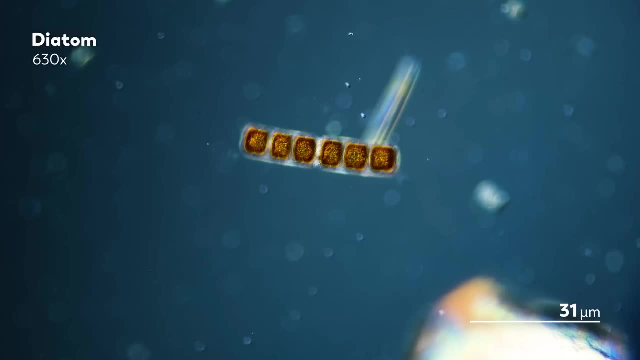 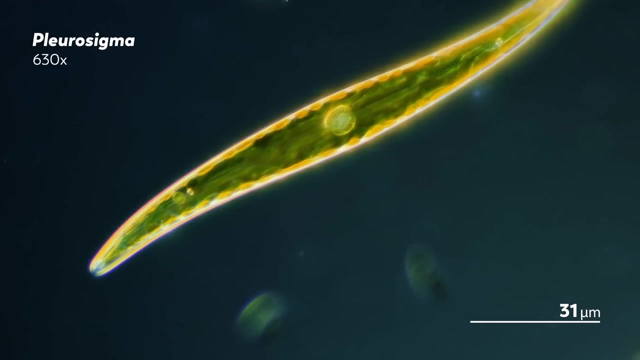 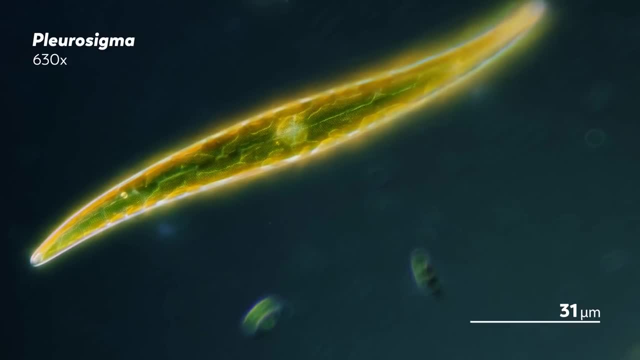 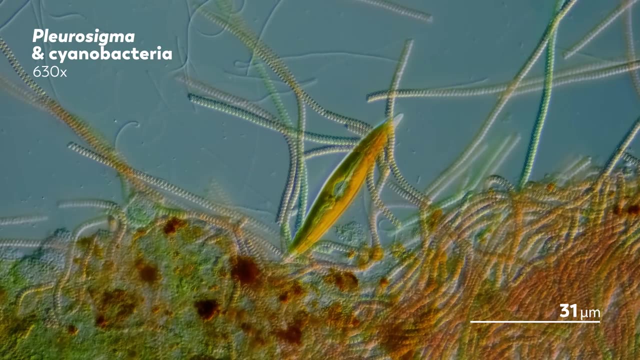 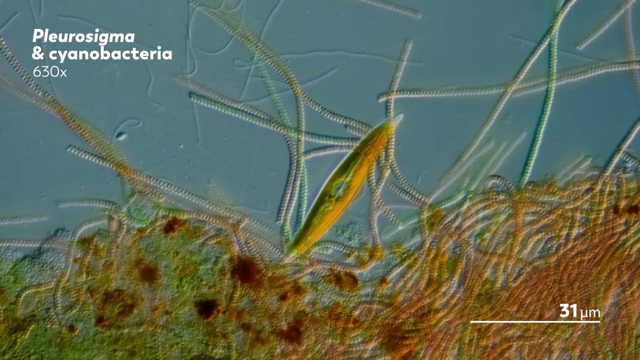 key assembly step, But there may also be other organic molecules — like proteins — that bind to the silica and help create the final structure. While scientists are still uncovering untangling those mechanisms, they have observed the way that the silica deposition vesicle and other structures in the cell, including the mitochondria. 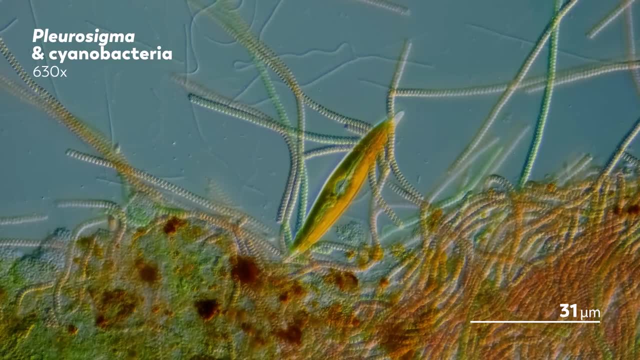 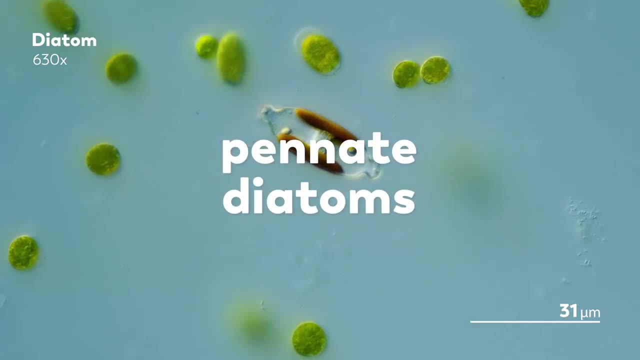 can help to mold the shape of the final silica structure. For example, elongated symmetric diatoms, also called pennate diatoms, often have a slit called the raphe. The slit helps the diatom move around, serving as an opening through which they can. 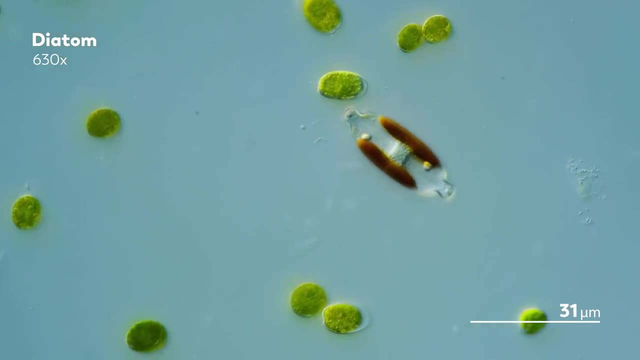 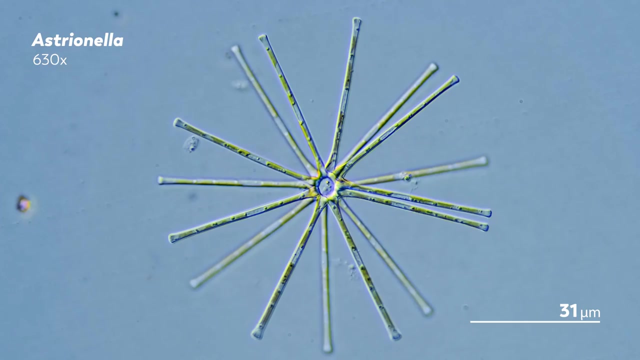 secrete a viscous fluid to glide on, And one of the ways that diatoms make the raphe is by physically molding it through the arrangement of their microtubules. Many diatoms are non-modal, meaning they don't move around And the lack of visible movement. 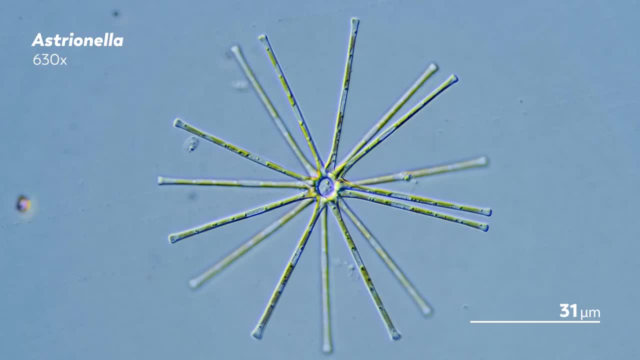 from the outside is striking when you consider all of the activity that has gone on inside of the diatom. So why do diatoms need to be molded to make those frustules happen? Like we said earlier, they're doing more than creating a smooth 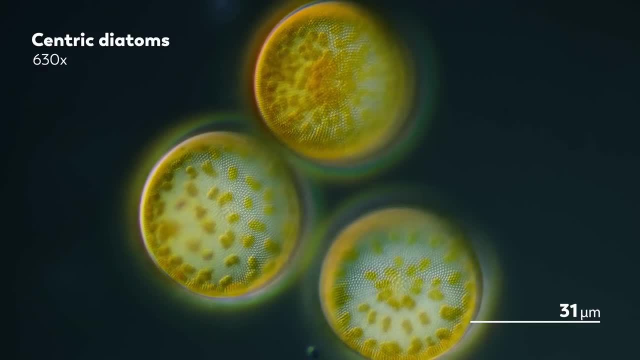 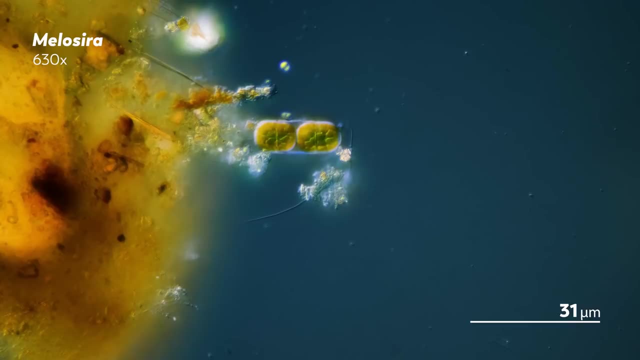 transparent surface. They're creating a molded, ornate structure personalized to their own shape, like a house couture. And not only is this process a lot of work, it renders diatoms dependent on silica, a chemical they can't make for themselves. 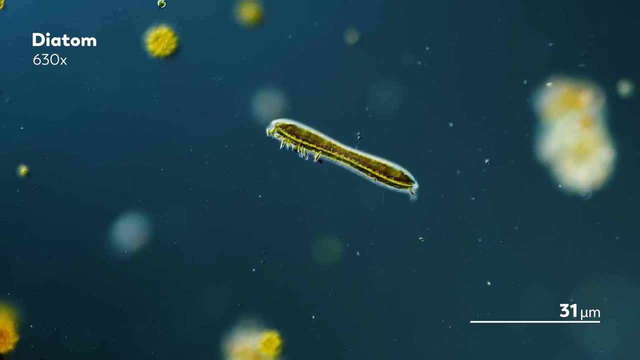 So why is this process a lot of work? Why do it? Well for one, it's cheaper than both making and assembling your own materials. Silica are already out there, so why not take advantage of it? One study found that materials in diatoms' frustules may help the organism take in carbon. 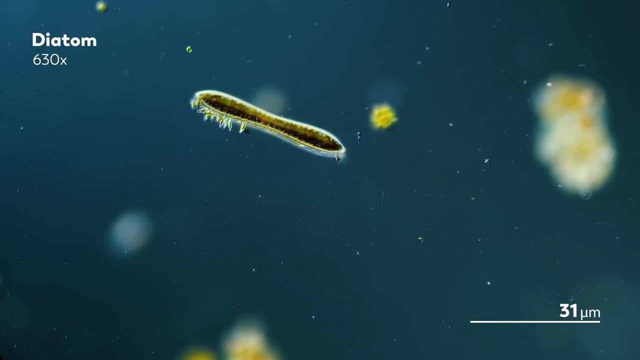 dioxide, improving their photosynthetic capabilities. These advantages seem to translate into the myeloma In different applications of charcoal. inserting in the first layer of cardboard, the metal layer is ain't like ah, howexciting. that still stays at once, because it's a little. buried and the fiber that is left remains unique and does no rotation at all. So we might even talk about the startup process in the future for diatom Rider, and with little respect, there you make a good deal at that. Those costs are unimpressive. 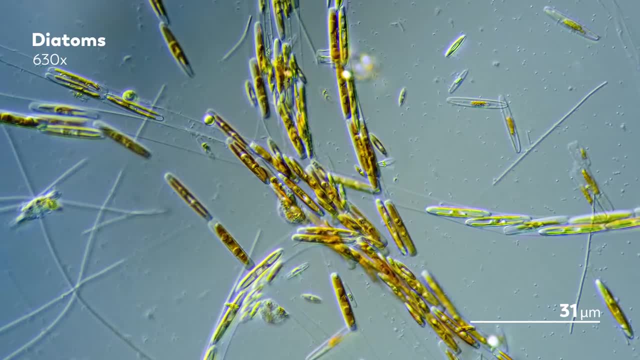 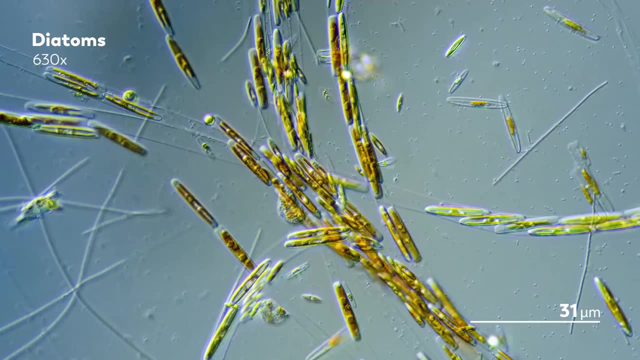 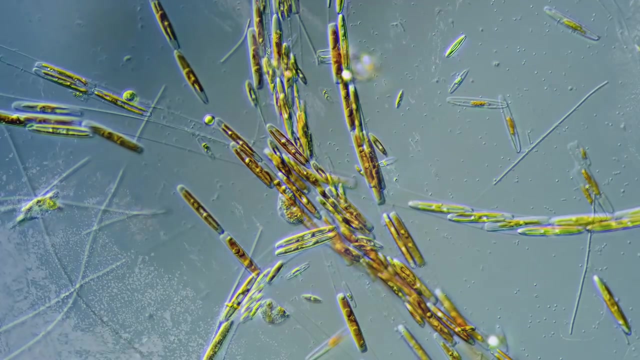 translate over into the immense capacity of diatoms to grow and dominate over other algae that share their waters. But taking over a body of water is all fun and games until the silica runs out. Diatoms are known for their ability to form large, visible blooms, whether in your local lake. 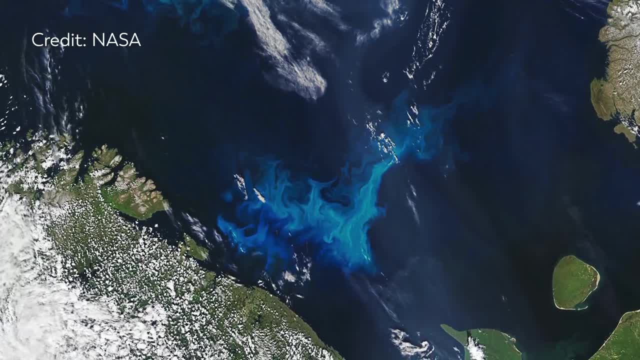 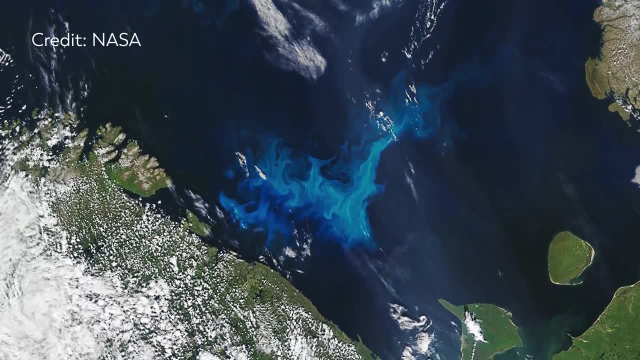 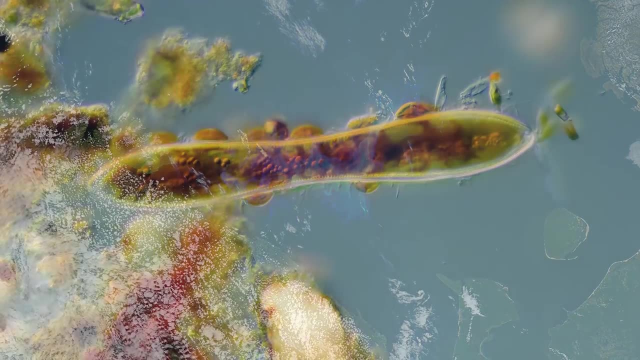 or the Arctic Ocean. But scientists studying those Arctic blooms found that as the diatom population expanded, they also depleted their waters of silicic acid And that in turn halted their growth and began to increase the number of dead diatoms. And both of these things. 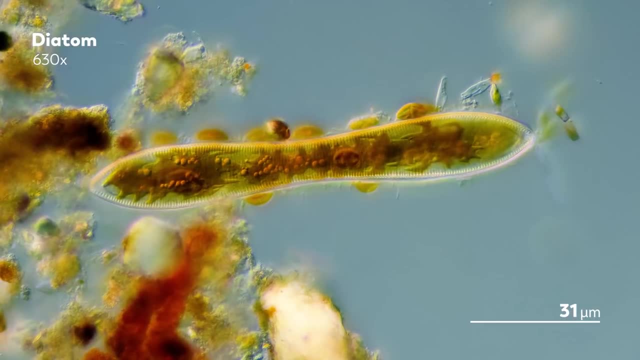 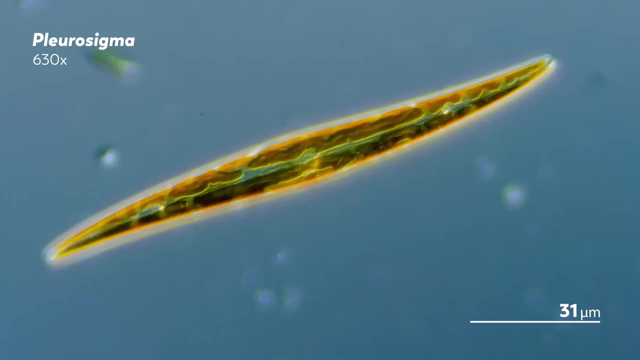 the lack of growth and the dying have another impact on diatom populations Sinking. Healthy, growing diatoms can up their buoyancy to keep them afloat, while dying cells cannot. It might be sad to imagine those blooms dying and descending to lower depths. 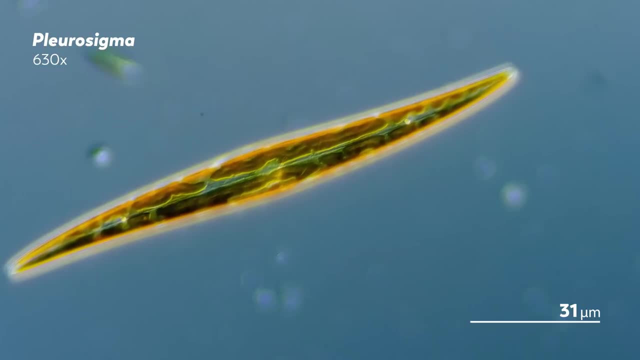 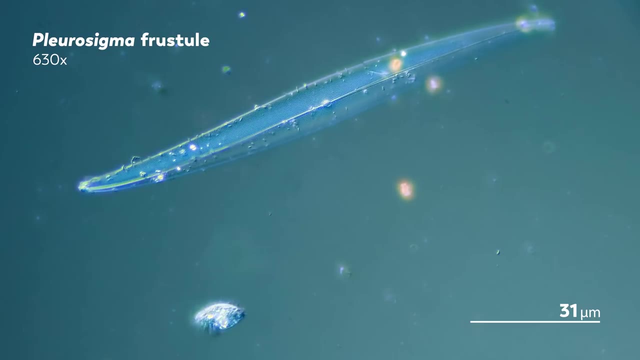 the ornate jewels collapsing like a microbial empire. But nature doesn't trade in inconsequential tragedies. The death of diatoms leaves behind frustules like this one, which means it leaves behind silica. Some of that silica can be recycled by other diatoms, but over time it will eventually. 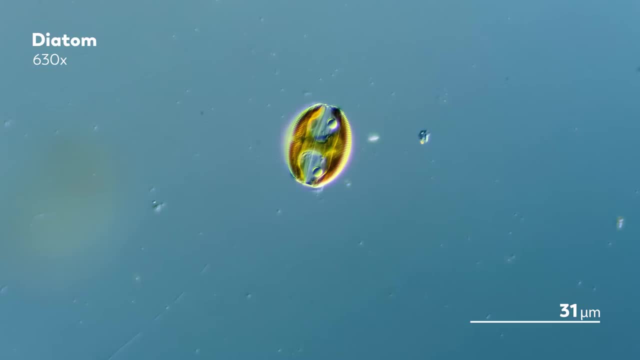 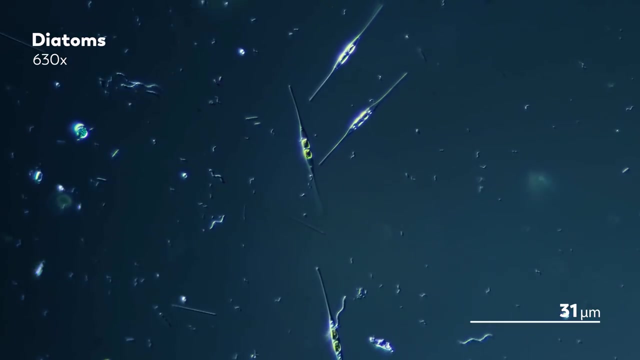 return to life as sediment. When a diatom takes in silicic acid, it takes in the remnants of a geological process, the weathering and erosion that brought the silicon to water in the first place, And then, through the construction of its shell, it recycles and transforms the 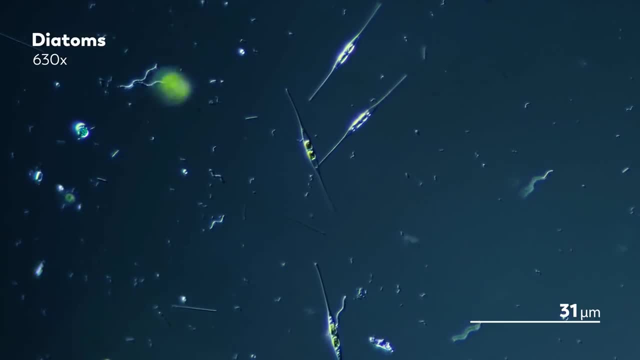 dissolved silicon into a form that can become geological once again. The chance of that silica being reused can vary, but as always, you can't be so sure with the diatom. Your your chances of running into it again are high. Scientists found that dust 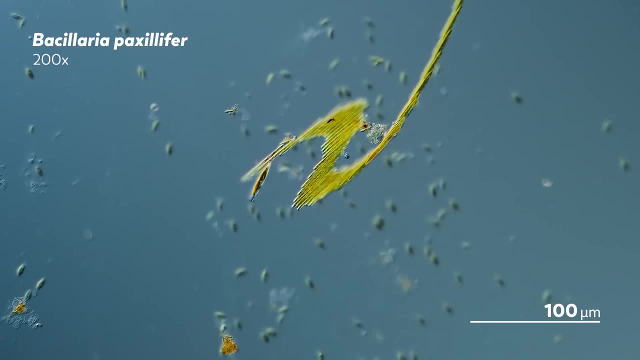 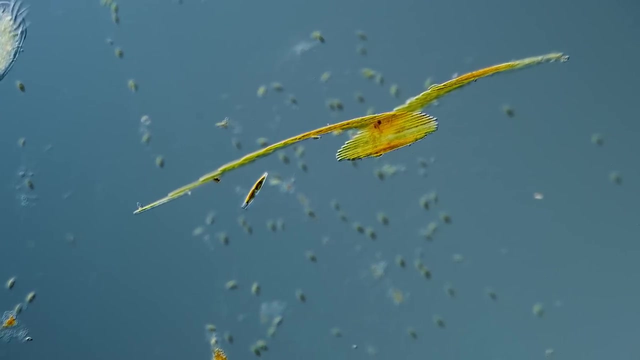 from a diatom shell-rich sediment in Chad might travel as far as the Amazon. The diatom itself may not be making the trip, but the microcosmos and the things built in it have a way of sticking around. Thank you for coming on this journey with us. 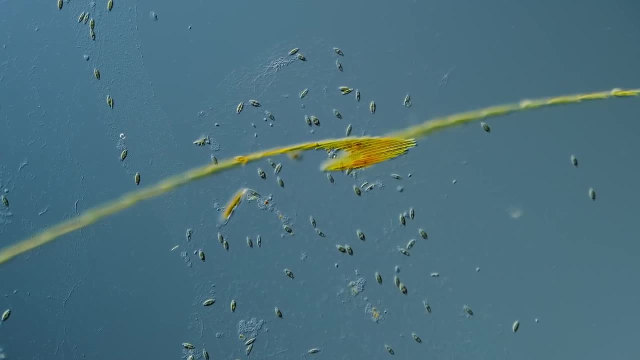 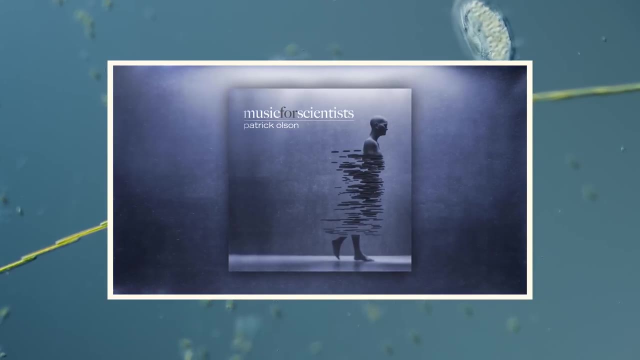 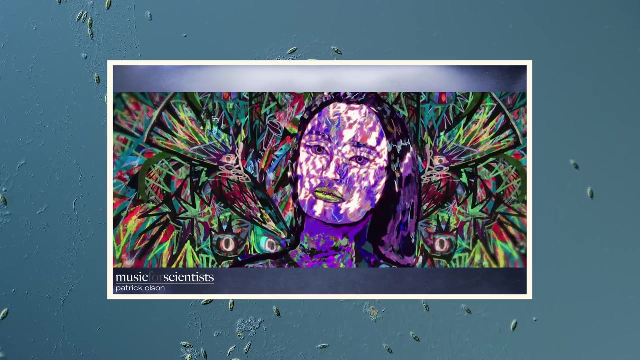 as we explore the unseen world that surrounds us. This episode is brought to you by the Music for Scientists album, which was created by composer and musician Patrick Olson. The album is inspired by the intersection of science and art, And if you're looking to explore that intersection more, 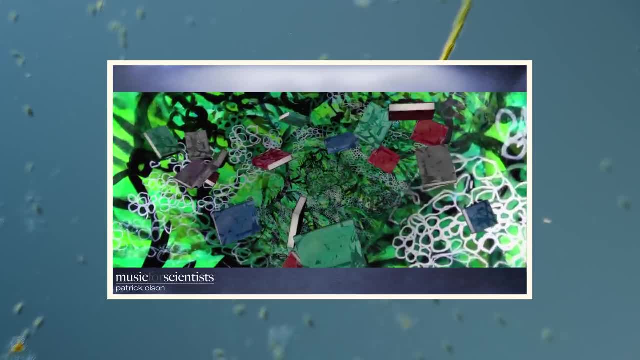 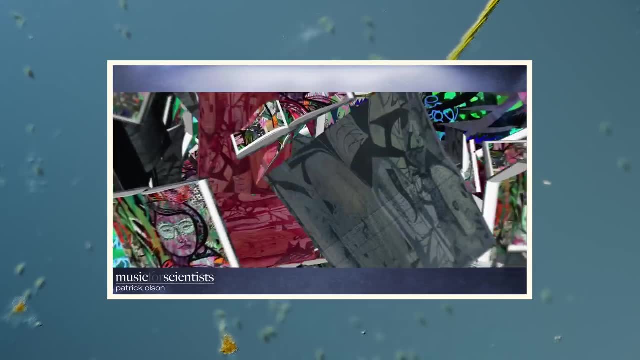 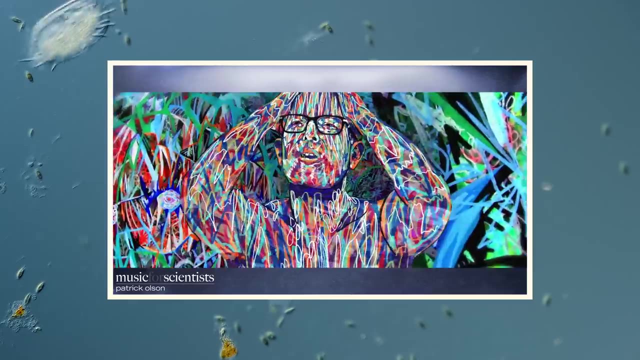 check out the music video for one of the tracks on the album called The Idea. The music video for this track was produced from a sequence of 15,000 photographs of three traditional paintings by artist John Todd. His painting style was then transferred to a video performance by using a form of machine learning. 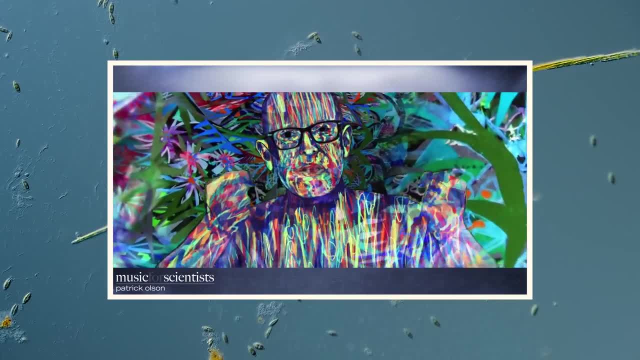 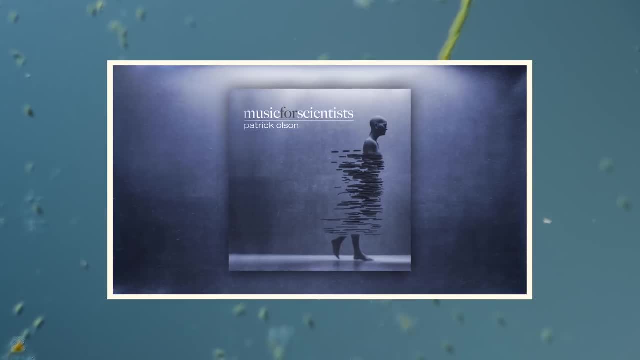 And the song itself is all about exploring how we form ideas. If you think this sounds like something you might enjoy, click the link in the description to see the video or stream the music on all major music services: The names on the screen right now. 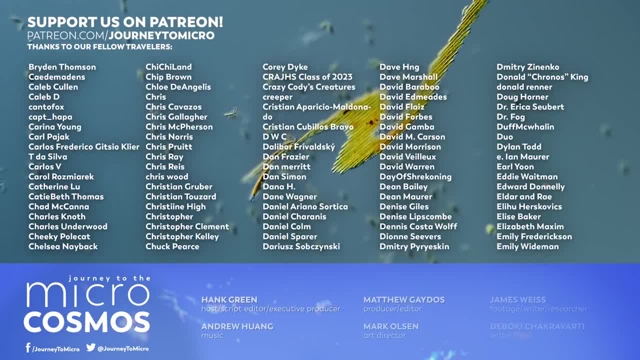 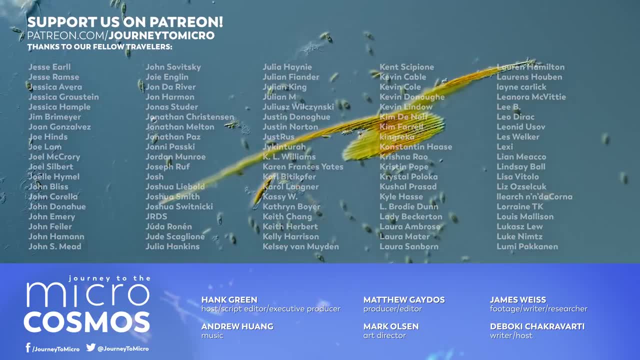 those are our Patreon patrons. Without them, we could not make this show and we are so thankful, Thankful to them. If you like what we do and want to help us keep making it, you can join those people at patreoncom slash journey to micro.